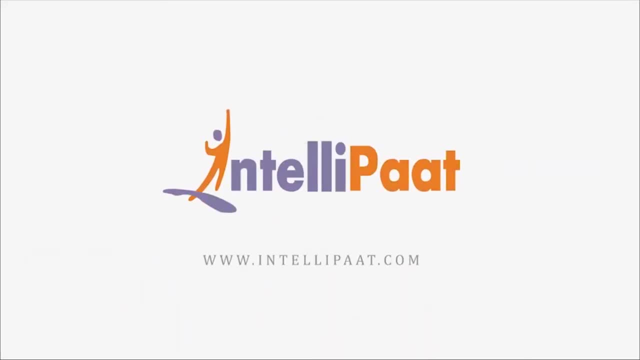 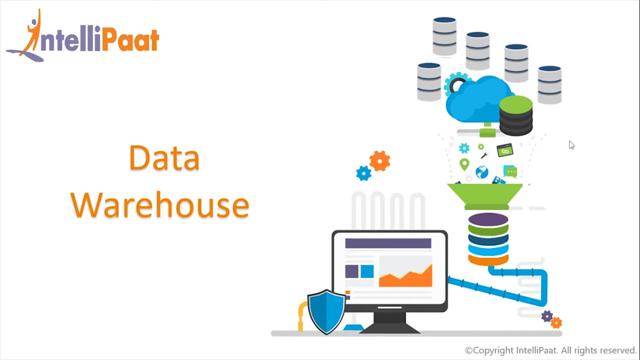 Hey guys, welcome to Intellipaat. This time we've come up with another exciting video on data warehousing. So you guys would have come across the term data warehousing but would have been unsure what exactly it is. So we've come up with just the right video to help you fully understand. 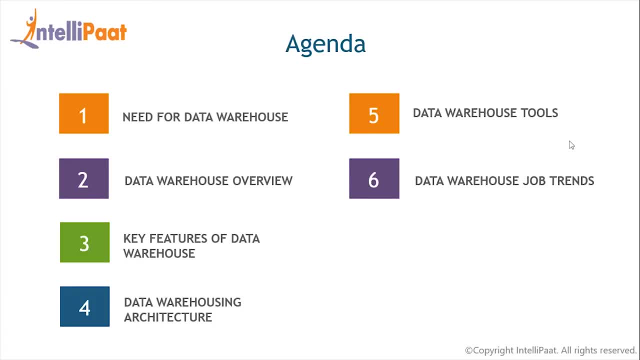 what data warehouses and what it can do. In this session, we will start off by understanding the need for a data warehouse. Then we'll understand what exactly is a data warehouse, and after that we'll look at the key features of data warehouse, Following which we'll discuss its architecture and 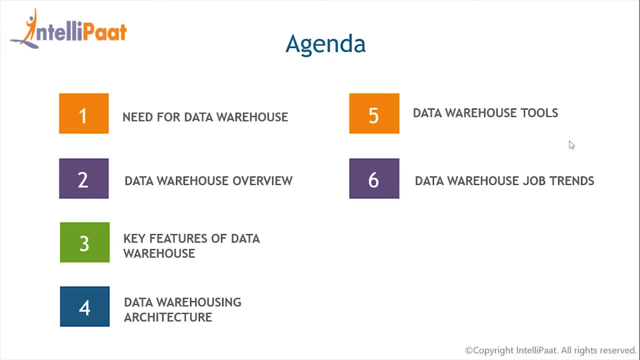 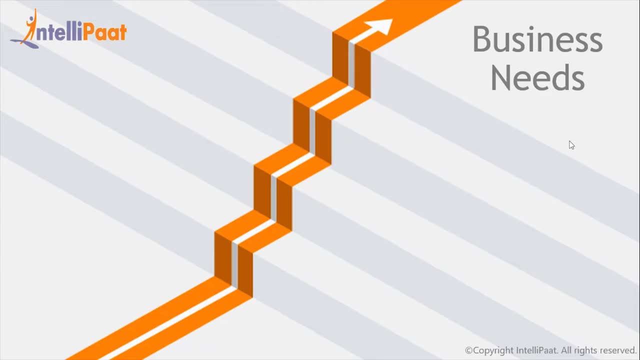 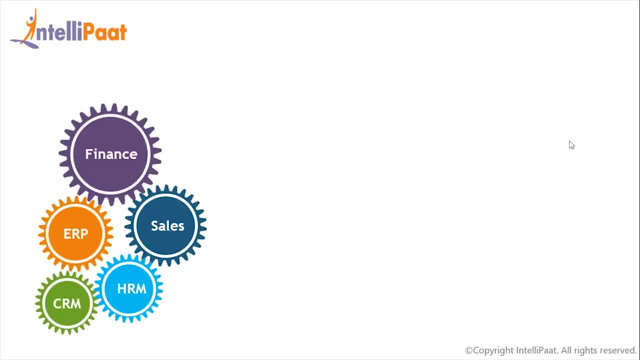 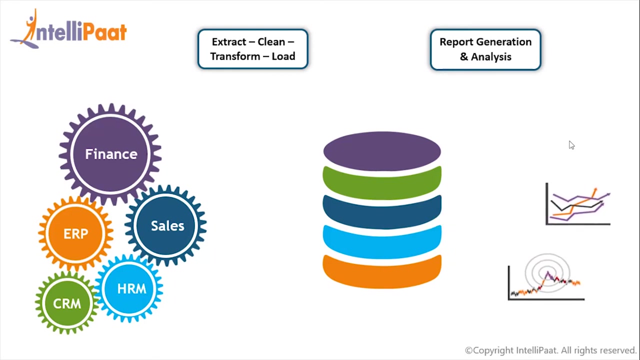 intelligence develops the ability to make better decisions. Business intelligence develops the ability to make better decisions. Business intelligence develops the ability to make better decisions. Business data warehouse will become the main source of information for report generation and analysis via reporting tools that can be used for things such. 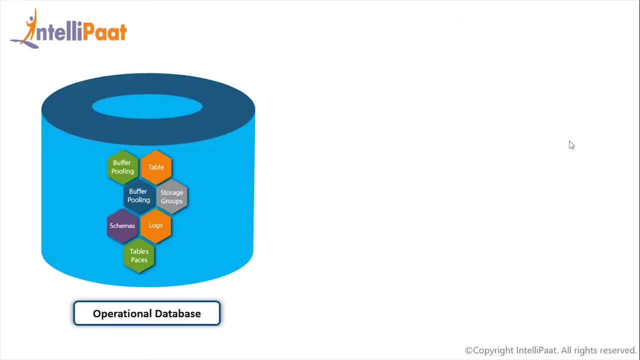 as ad hoc queries and dashboards. Now, sometimes it has been noticed that many companies say they have a data warehouse, but they don't really have a true data warehouse. Rather, it is actually a dumping ground for tables that are copied from source systems with little modification. So for a company to be 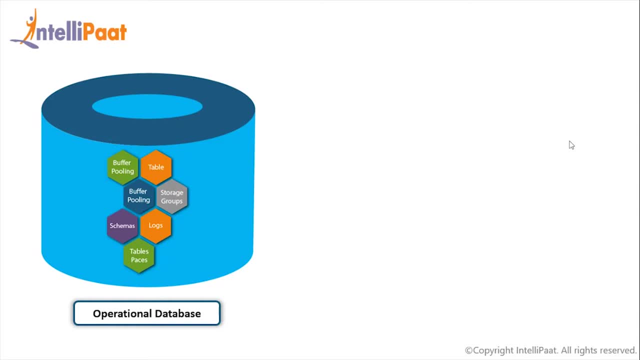 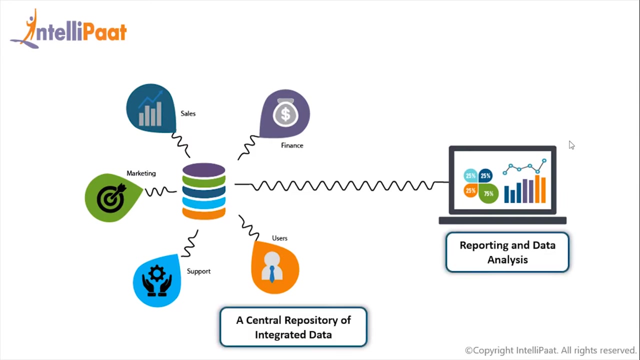 successful in future, they must make good decisions, and to make good decisions, they require all relevant data to be taken into consideration, And the best source for that data is a well-defined data warehouse. So a data warehouse is specially designed to perform business intelligence activities and enables professionals and employees to comprehend and improve the 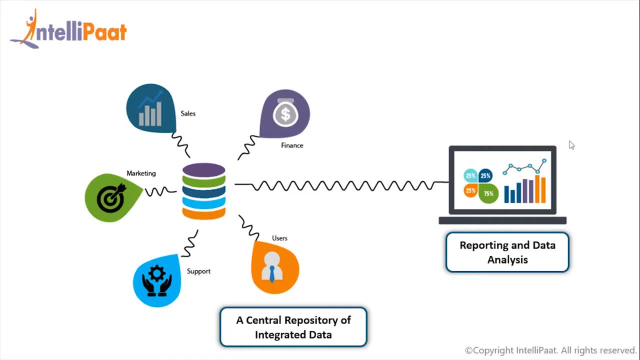 organization's overall performance, And the two major functions of a data warehouse are to make sure that the data is being processed in a way that is maintained- past and present records- and also help organizations to take effective business decisions with precise data analysis. Additionally, the data warehouse environment also supports ETL data mining capabilities. 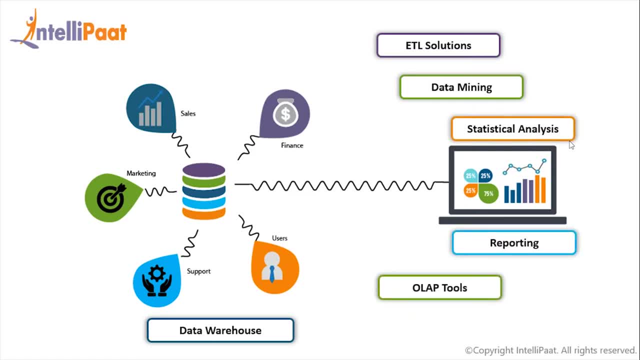 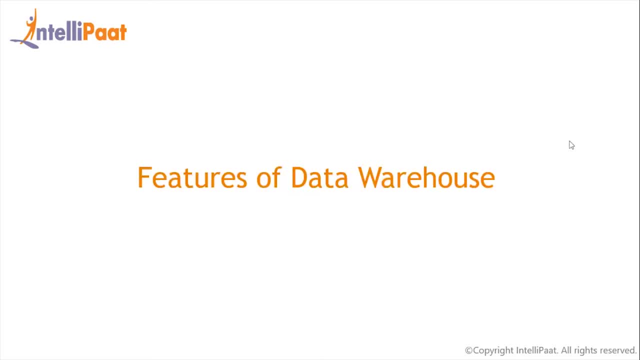 statistical analysis, reporting and OLAP tools which help in interactive and efficient data analysis in a multi-faceted view. Now we'll look at some of the key features of data warehousing. So number one in the list is subject-oriented. So data warehousing gives you an option to analyze a 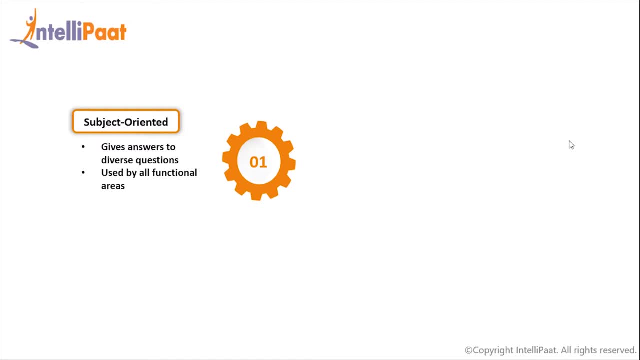 particular subject area. Thus a subject matter expert can answer relevant questions from the data. For example, if that particular subject is sales, then a sales executive for an online website can develop a subject-oriented database including the data fields he wants to query, So the salesperson can extract. 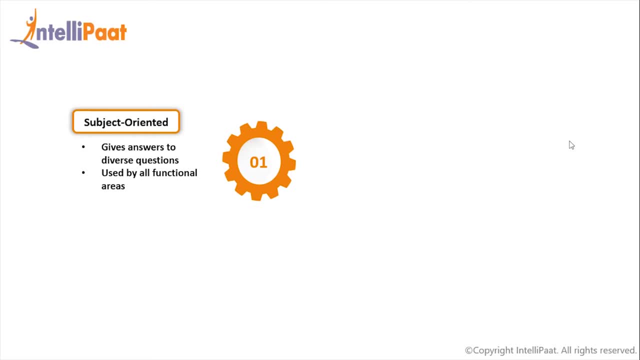 data writing. different queries like how many customers purchase the data based architect course today And next in the list, is integrated. So a data warehouse supports consistency by arranging data from diverse sources in a uniform and rational format, So it should not allow any conflicts in the field. 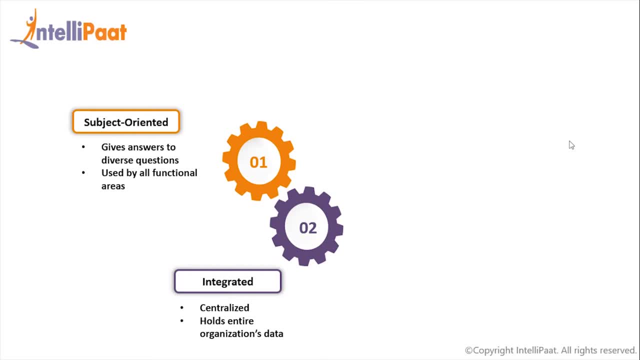 names and other units of measure. Having accomplished the studiness, we can refer it to be an integrated warehouse. The third key feature is non-volatile. So, as the name suggests, nonvolatile data warehouse refers to no data change once you download review file and download a document to 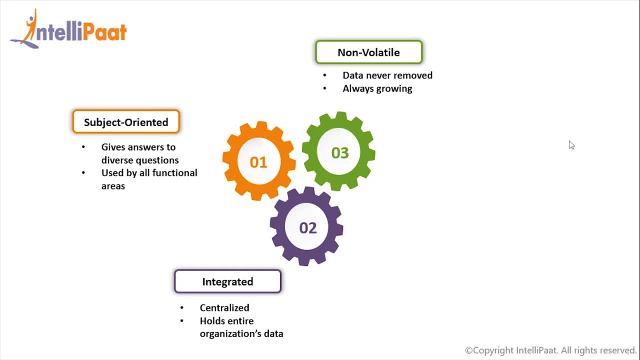 created. It is an important and relevant feature, since the aim of developing a warehouse is to evaluate what has occurred until then. And the fourth key feature is time variant, So the data collected in a data warehouse is identified with a particular time period, So this data provides information from 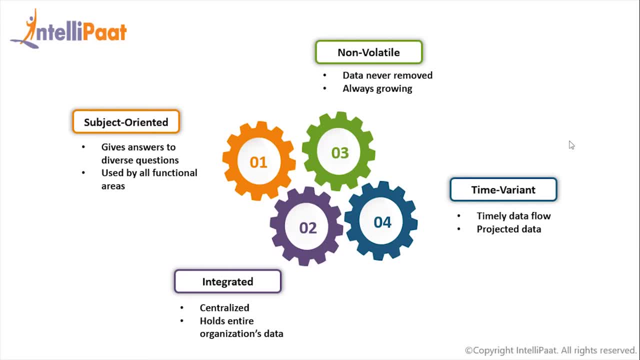 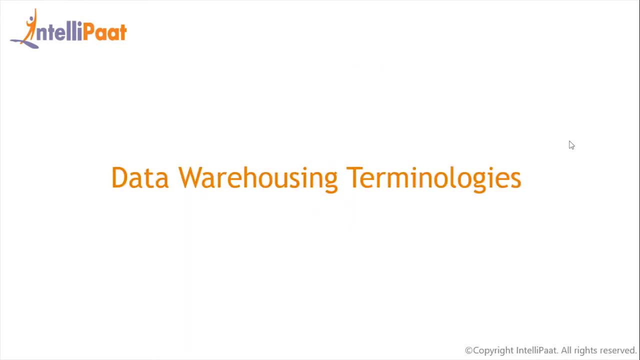 the historical point of view. For example, one can retrieve data from the past 3 months, 6 months, 12 months or even older data from a data warehouse. So now we'll look at some of the most frequently used terms in data warehousing. We'll start. 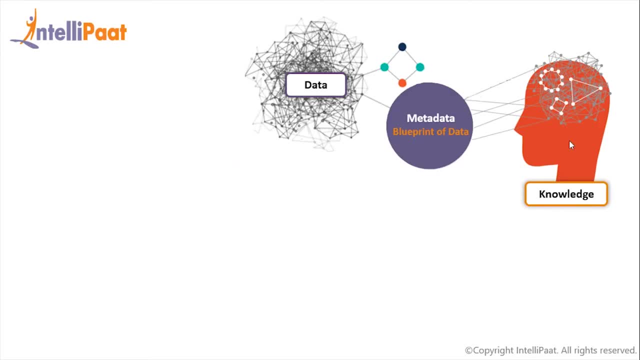 with metadata. In simple terms, metadata provides the answers to all your data related questions. in the data warehouse It is referred as data about data, So it gives users a detailed explanation of the syntax and semantics and describing all relevant attributes of the data in the data warehouse. 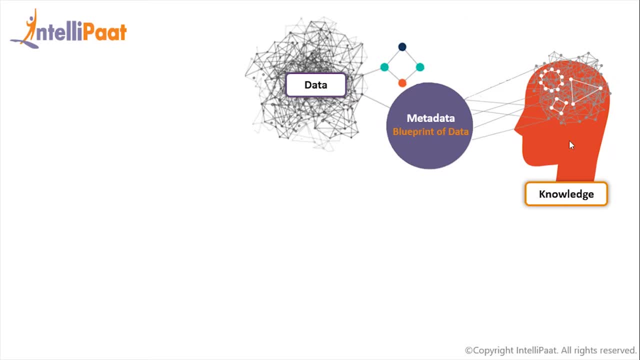 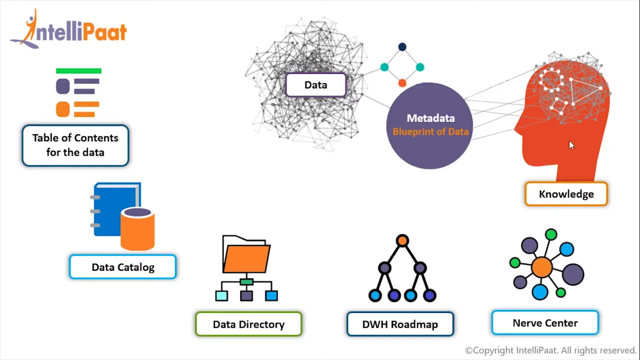 For instance, the number of tables in a database can be referred as metadata. Now the metadata is also commonly known as table of contents for the data, data catalog, data directory, data warehouse, roadmap and the nerve center. So, with the help of metadata, developers and database administrators can create their own. 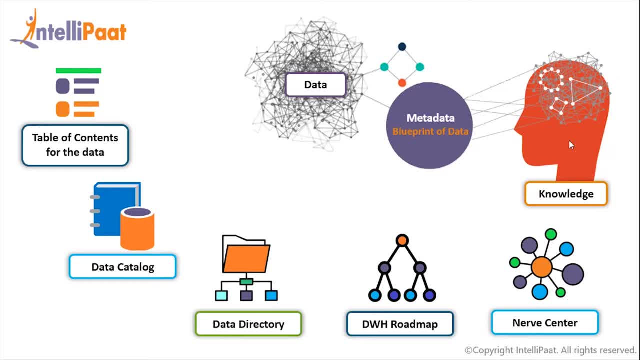 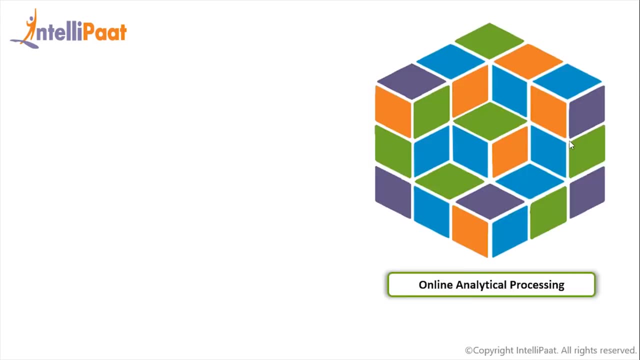 ad hoc reports, which is of prime significance in this era of big data. In fact, without metadata, the data warehouse can be called metadata, So the metadata is considered futile. It would just be a big box without any valuable and meaningful information. Then we have OLAP, which expands to online analytical processing. 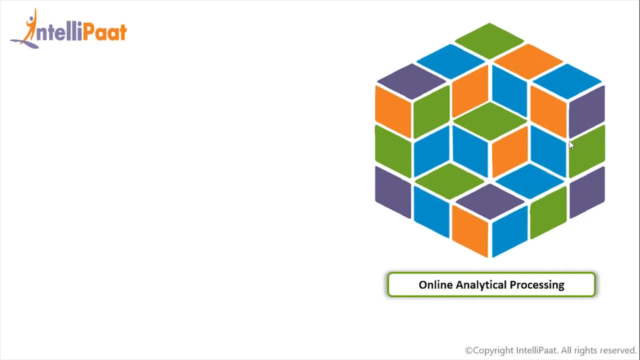 As the name suggests, OLAP is computer processing which allows users to interactively analyze multi-dimensional data from multiple prospects. The various techniques of multi-dimensional model of OLAP constitute and encapsulate large volumes of data for rapid evaluation In a multi-dimensional environment. each attribute of data is considered a separate 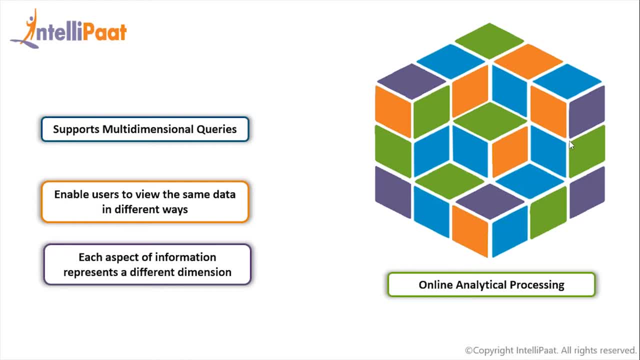 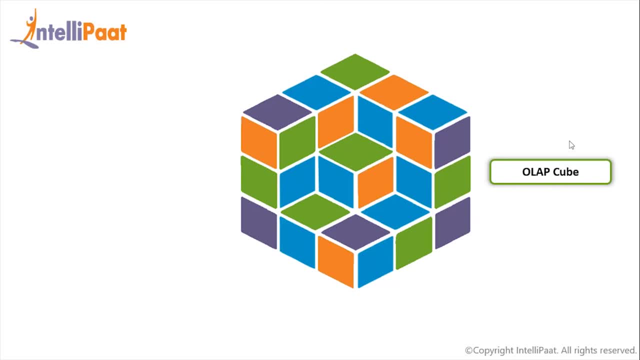 dimension, and OLAP can establish an intersection between these dimensions. So the OLAP cube is typically similar to the shape of a cube and it has the multi-dimensional representation of data which is optimized for data warehouse. It is an array or matrix of facts and dimensions, wherein a fact table contains facts or metrics. 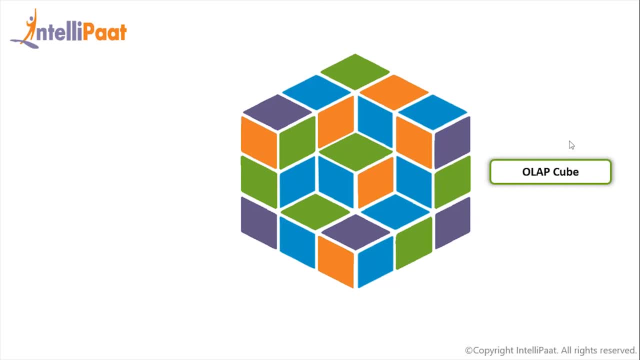 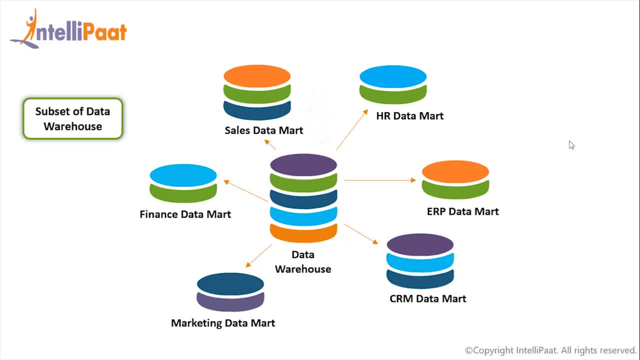 The fact table contains the facts or metrics of the data warehouse. The fact table contains the facts or metrics of the data warehouse. The fact table contains the facts or metrics of data warehouse, which is aligned to a specific business perspective. While a data warehouse stores detailed information of multiple subjects, the 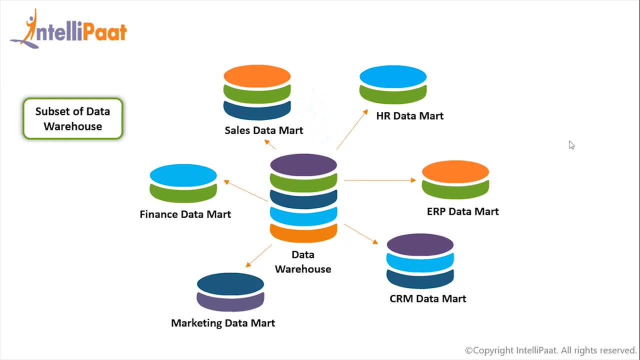 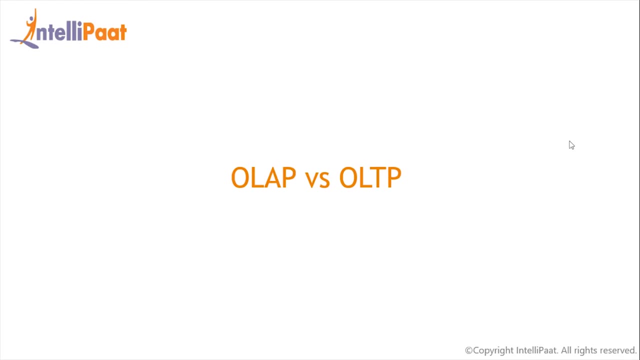 latter focuses on storing data about only one subject, and the data mart concentrates on storing more summarized form than complete data and integrating information within specific set of source systems. Now let's move further and discuss some of the major differences between OLAP and OLTP. 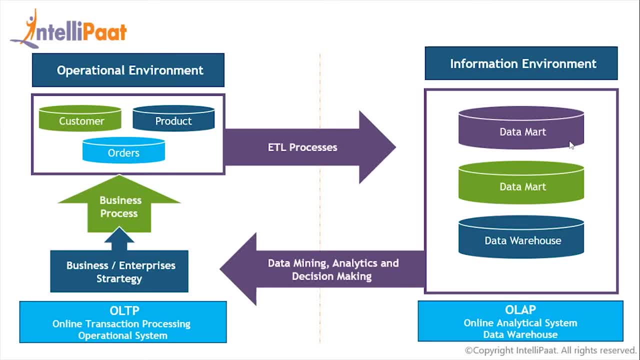 Generally, people get confused with OLAP and OLTP. They are two different types of data analysis techniques and are distinct from each other in many ways. So here on the screen we see the collaboration between OLTP and OLAP In this workflow architecture. we can depict the importance of each. 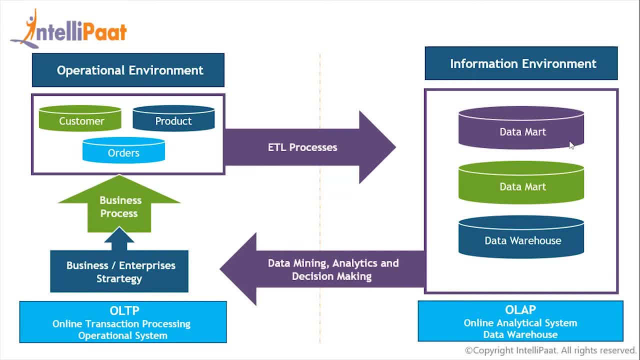 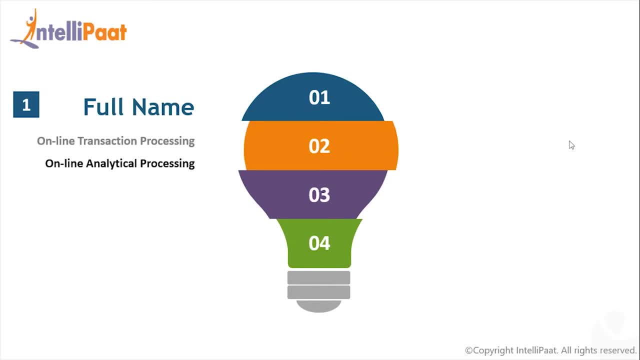 system-based application and how they are linked with each other. The first difference is the name itself: OLTP stands for online transaction processing, while OLAP stands for online analytical processing. The main difference between them is that OLTP focuses on small transactions and faster query. 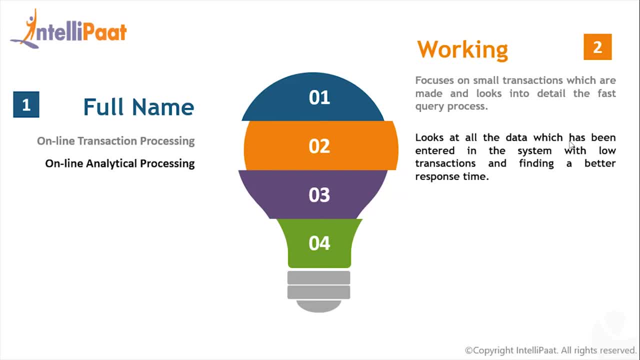 process. OLAP, on the other hand, often involves complex queries involving aggregations. Another difference between them is that the data for OLTP is mostly operational, while for OLAP it has consolidated data which comes from various OLTP databases, and OLTP system shows an image of all the activities. 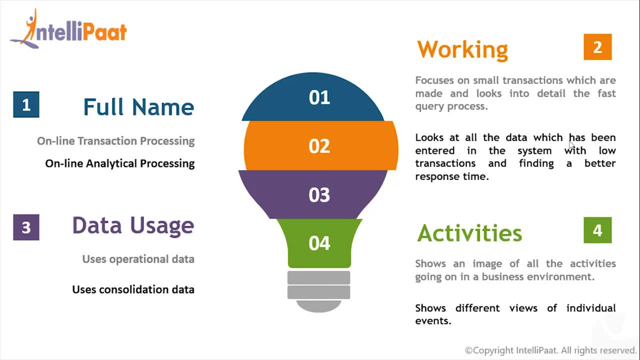 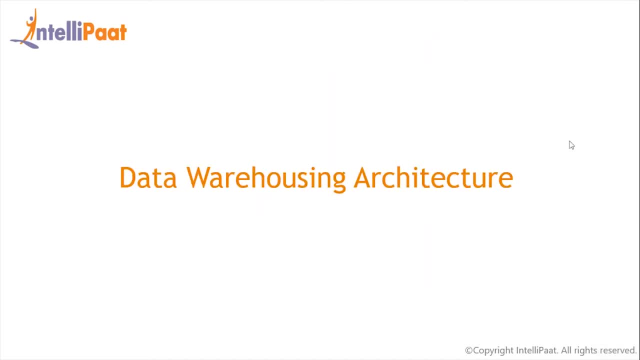 going on in a business environment, while OLAP system shows different views of individual events. Now that we've understood the concept of data warehouse, it's time to gain some insights into the architecture of data warehouse. So there are two main components. So there are two main components. 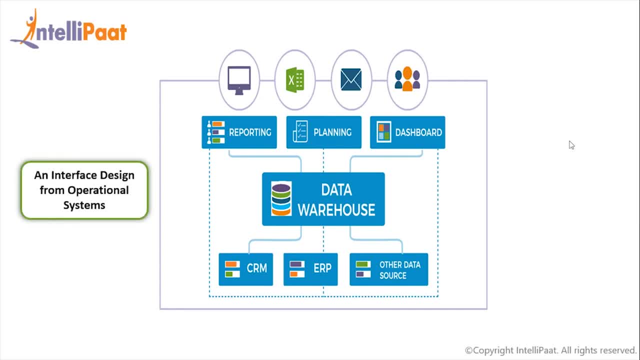 to building a data warehouse, An interface designed from operational systems and the individual data warehouse design. Thus, the construction of data warehouse depends on the business requirements, where one development stage depends on the results of the previously developed phase. The structure of a data warehouse can be understood better through its layered model, which 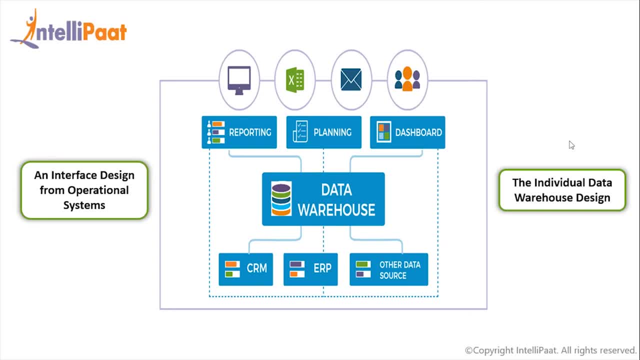 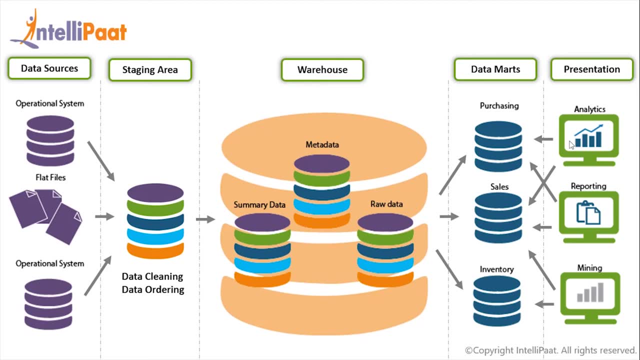 lists all the main components of the data warehouse architecture. So here is a typical architecture of data warehouse consisting of different important components. You can see that it is nothing but the movement of data from source to the staging area and then finally to the confirmed data match. 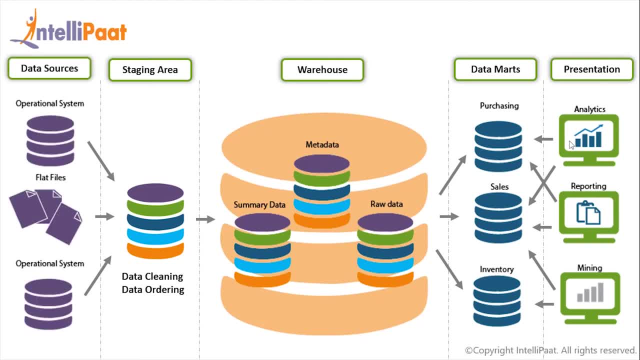 through ETL. The first layer is the data source layer, which refers to various data stores in multiple formats, like relational database, excel file and others. These stores can consist of different types of data, such as business data, web server logs and internet data. 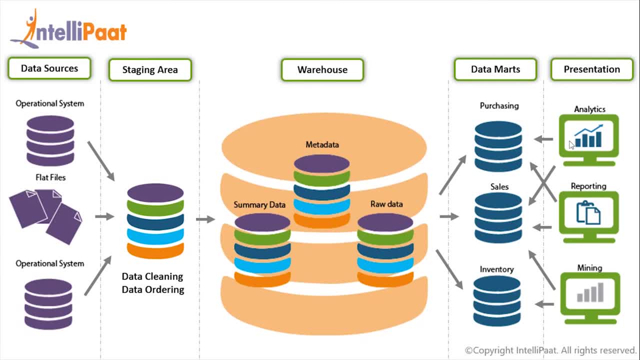 The next step is extract, where the data from data sources is extracted and put into the warehouse staging area. This extracted data is minimally cleaned with no major transformations. Then comes the staging area, which is divided into two parts: data cleaning and data ordering. So as 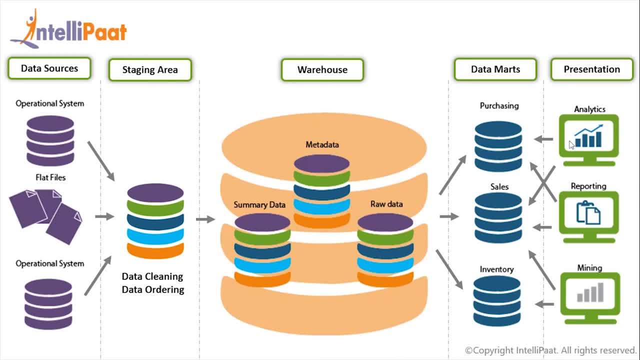 the name suggests, this layer takes care of data processing methods, Thus removing data redundancy, filtering bad data and proper operation of data Overall. this stage allows application of business intelligent logic to transform transactional data into analytical data. It is indeed the most time-consuming phase in the whole data warehouse. 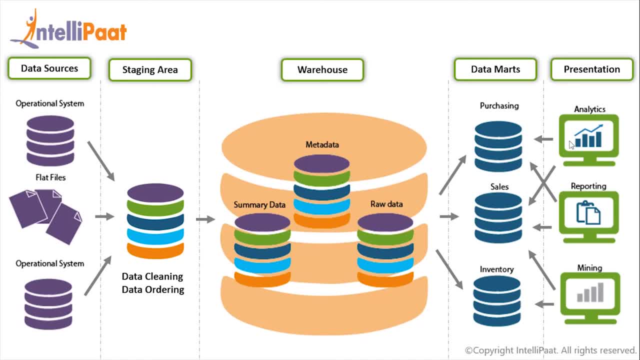 architecture and as the chief process between data source and presentation layer of data warehouse. Finally, we have the data presentation layer, which is the target data warehouse, The place where the successfully cleaned, integrated and transformed data is stored in a multi- dimensional environment. Now the data is available for analysis and query. 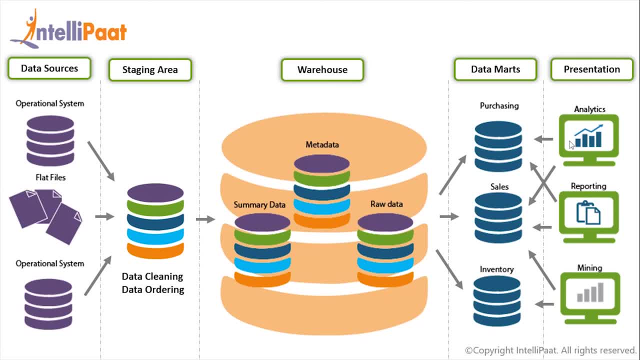 purposes. The information is also available to end users in the form of data marts. This data can then be accessed by various business intelligence tools like tableau, and presented in multiple formats like tables, graphs and reports. It is important to note that the data warehouse supports and holds both the 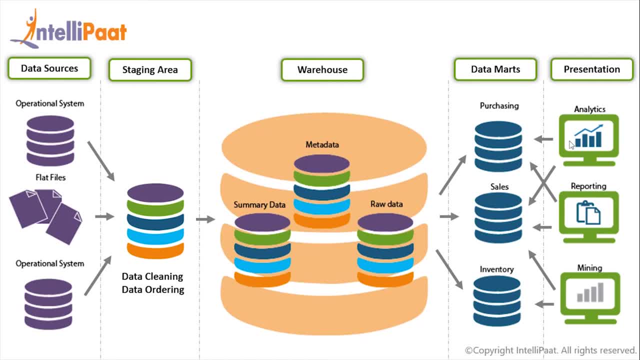 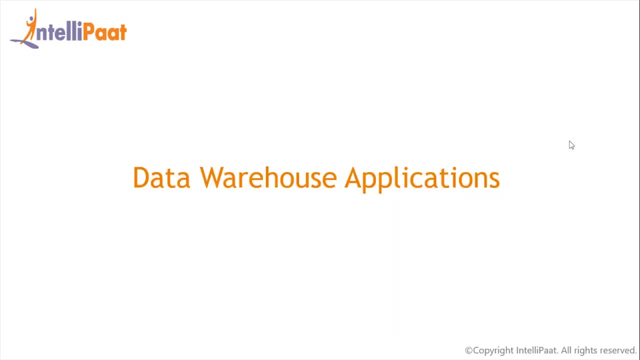 persistent data that is stored for longer time, and also temporary data. The major purpose of a data warehouse is the attainment of cleansed, integrated and properly aligned data so that it is easy to analyze and present to clients and customers in several businesses. Now we'll understand for what purpose data 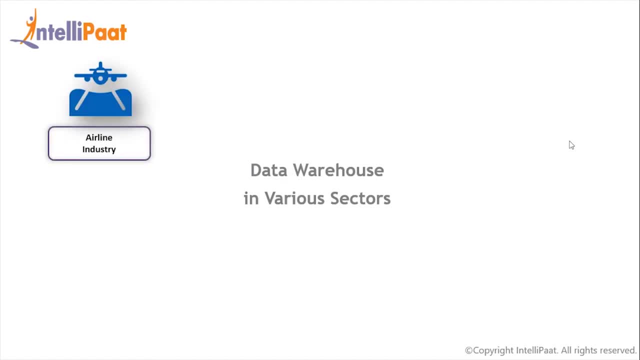 warehouse is used in various sectors. In the airline industry it is used for operation purpose, like crew assignment, analysis of route profitability and frequent flyer program promotions. In the banking sector, it is widely used to manage the resources available on desk Few. banks also use data warehousing. 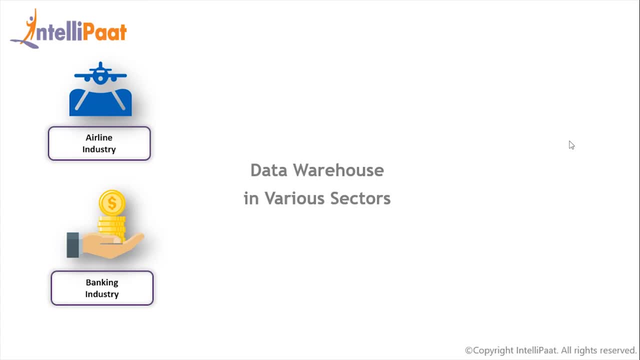 for market research, performance analysis of the product and operations. Healthcare also uses data warehouse to strategize and predict outcomes, generate patients treatment reports and medical aid services In the public sector. data warehouse is used for intelligence gathering. It helps government agencies to maintain and analyze tax records and health policy records for every. 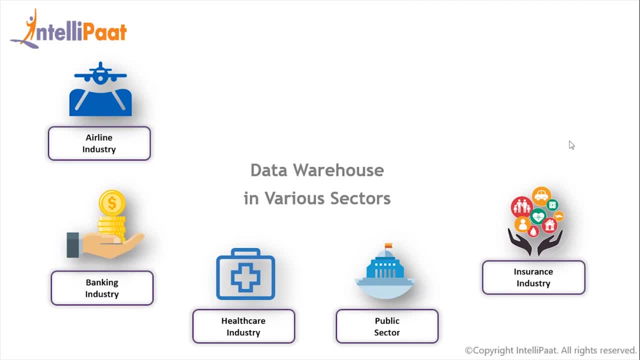 individual. In investment and insurance sector, the warehouses are primarily used to analyze data patterns, customer trends and to track market movements. In retail chains, data warehouse is widely used for distribution and marketing. In telecommunication, data warehouse is used for product promotions, sales decisions. 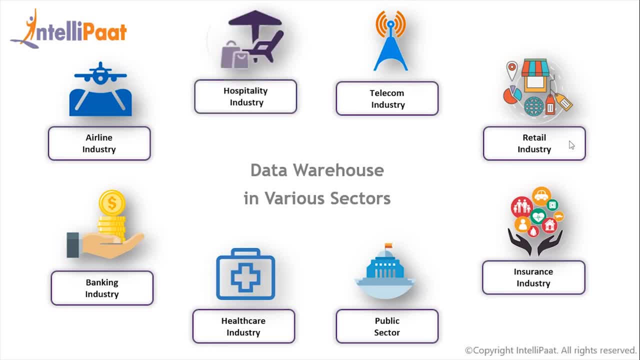 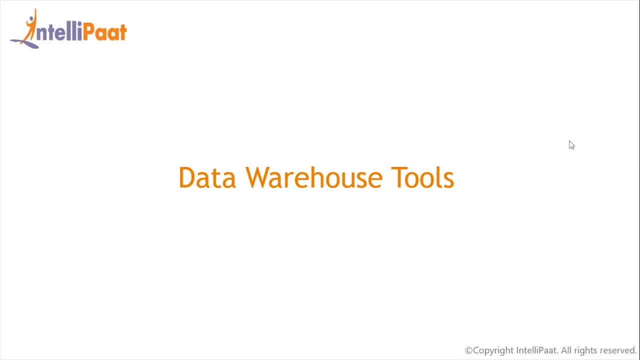 and to make distribution decisions. The hospitality industry utilizes warehouse services to design as well as estimate their advertising and promotion campaigns, where they want to target clients based on their feedback and travel patterns. Now there are many data warehousing tools available in the market. Let's have a look at some of the prominent ones. So Oracle is the